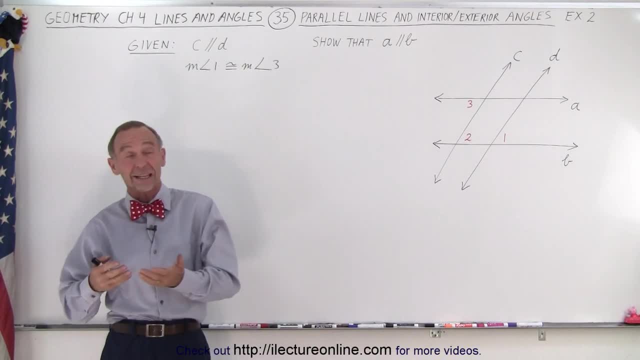 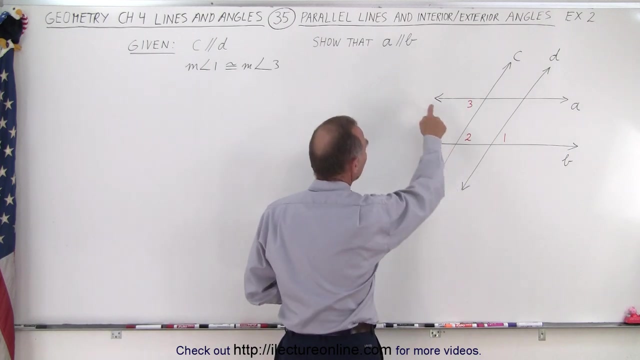 Welcome to our lecture online. So here's a second example, trying to determine if two lines are parallel, based upon what we know about interior and exterior angles. So here we're, given two pairs of lines. We have given C and D and A and B, and they told us that. 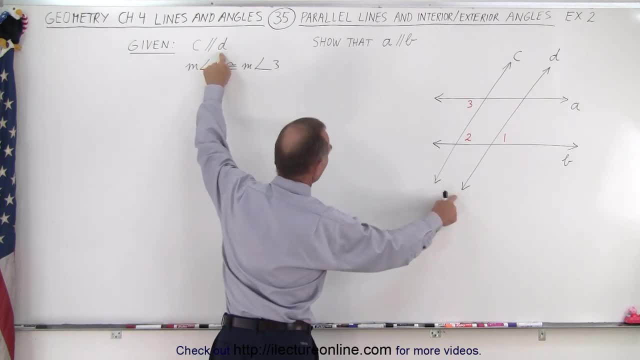 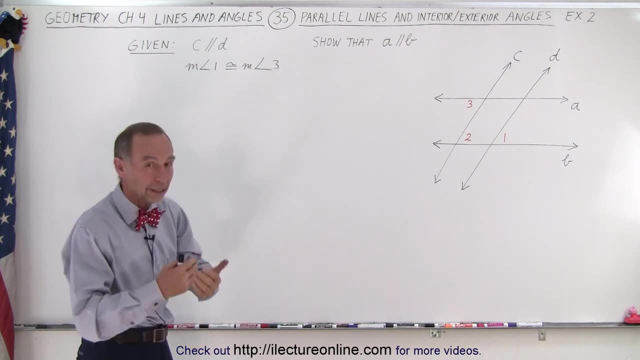 C is parallel to D, So these two lines are parallel to one another. They also told us that the measure of angle one is congruent to measure of angle three, So angle one and angle three are congruent. Now we're supposed to show that lines A and B are parallel to. 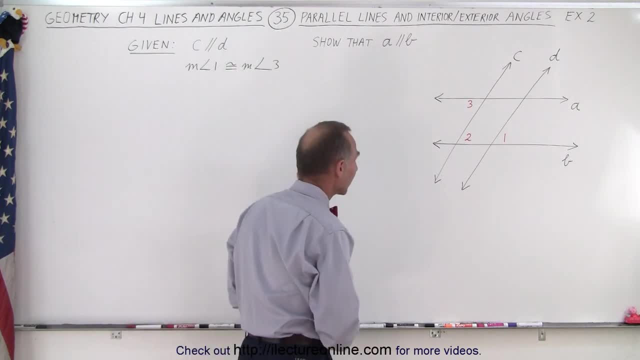 one another. So first of all, let's mark what we have here. We can see that this angle right here is congruent to this angle right there. So I have to find some information about these angles here in order for me to determine if A and B are parallel. 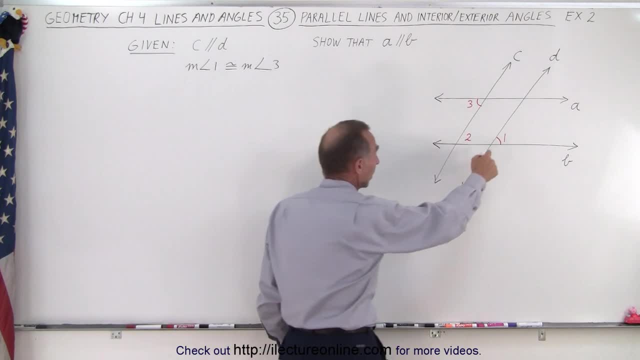 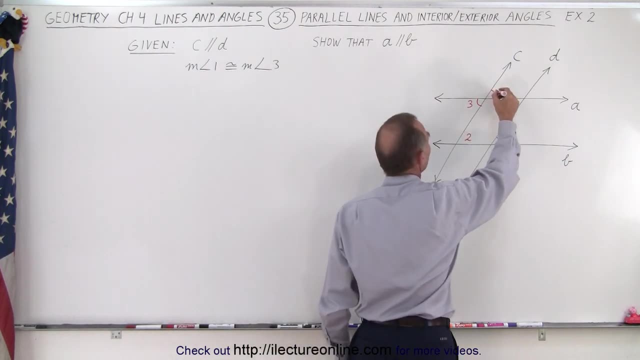 Because I don't know anything about angle two, so I do have to work out for these two angles right here. But then I realize that vertical angles are congruent, which means that this angle here is congruent to this angle right there. So let's call that angle. 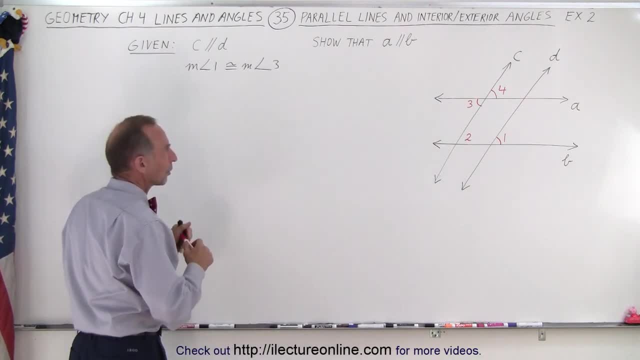 four. And so we know that angle three and angle four are what we call vertical angles or opposite angles. And so we can say that angle three and angle four are vertical angles, And from that I can conclude that they must have the same measure. So therefore we can. 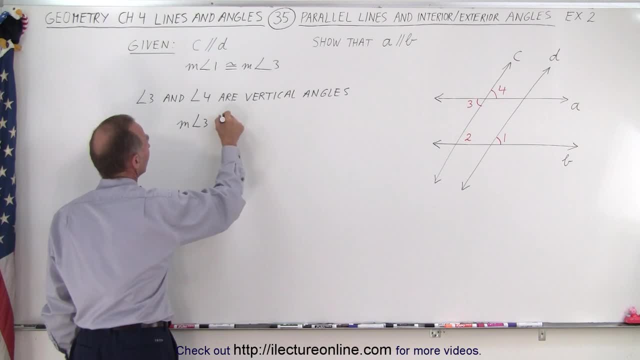 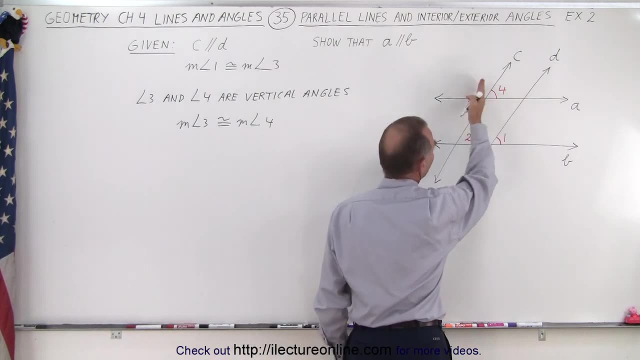 say that the measure of angle three is congruent to the measure of angle four. Alright, so now we know that C and D are parallel, And this is an interior angle, right here, And this is an interior angle. These are what we call corresponding interior angles, if we assume. 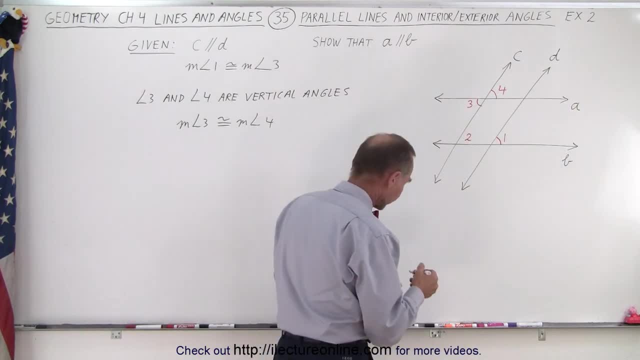 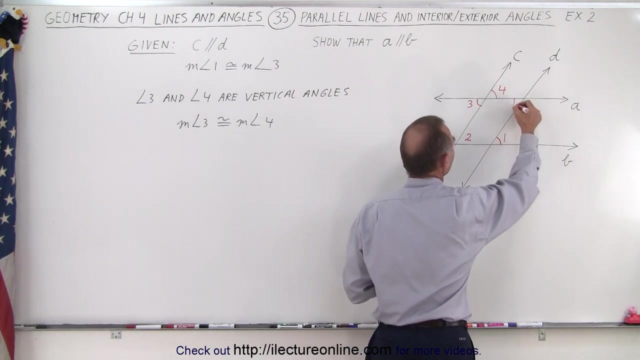 that line A is the cuts through angles C and D, And so therefore, we know that angle four must therefore be, that's, an interior angle, must therefore be congruent to this angle right here. So let's call this angle angle five. And so we know that they must be congruent, because this is